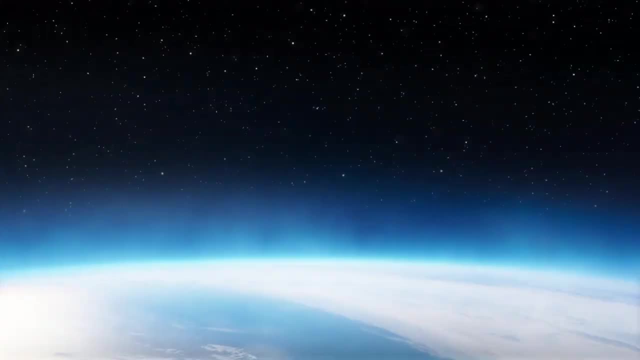 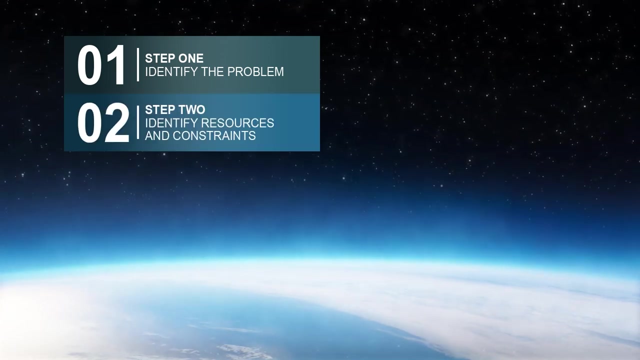 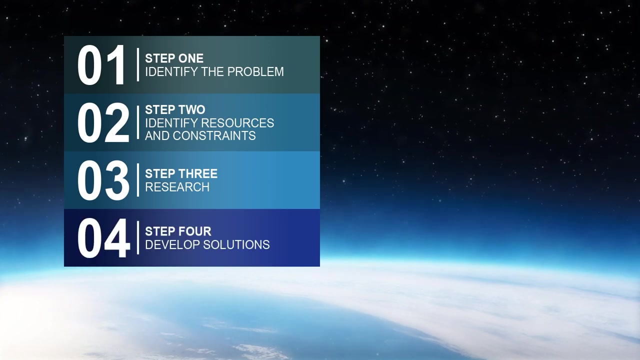 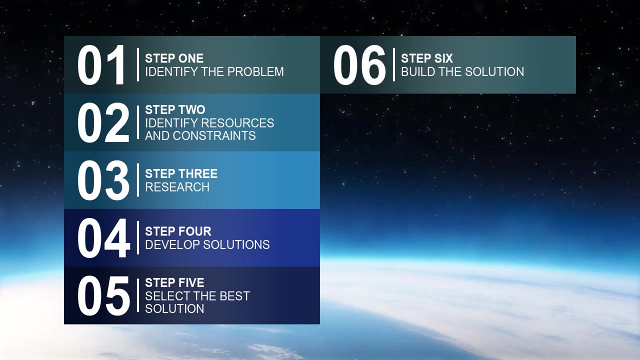 Here's one example of what the process looks like: Step 1. Identify the problem. Step 2. Identify resources and constraints. Step 3. Research. Step 4. Develop solutions. Step 5. Select the best solution. Step 6. Build the solution. 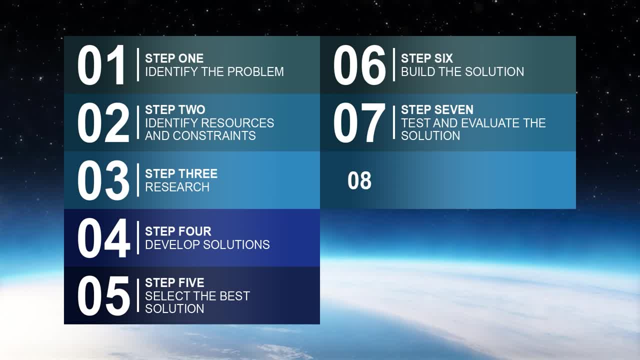 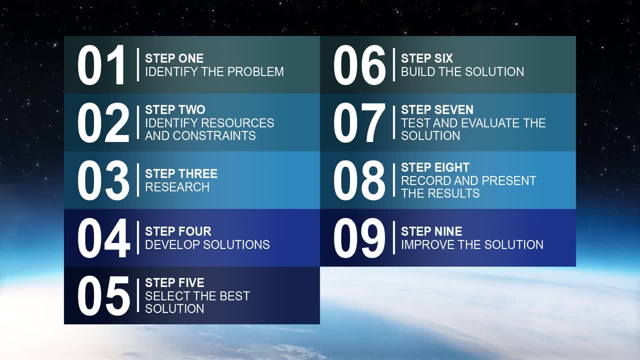 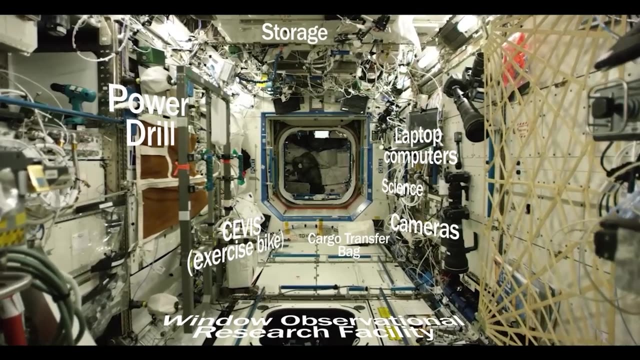 Step 7. Test and evaluate the solution, Step 8. Record and present the results. And Step 9. Improve the solution. Take a look at the space that we are currently living and working in. This space is filled with things that have been engineered using the engineering design process. 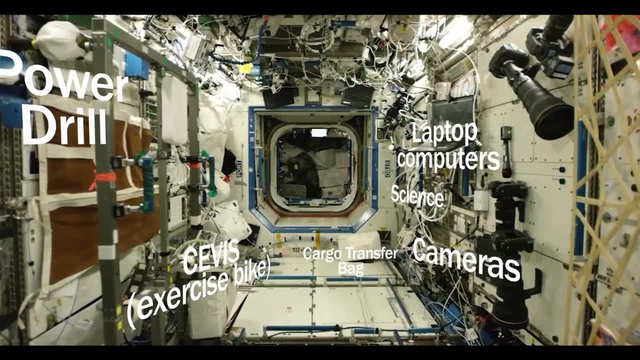 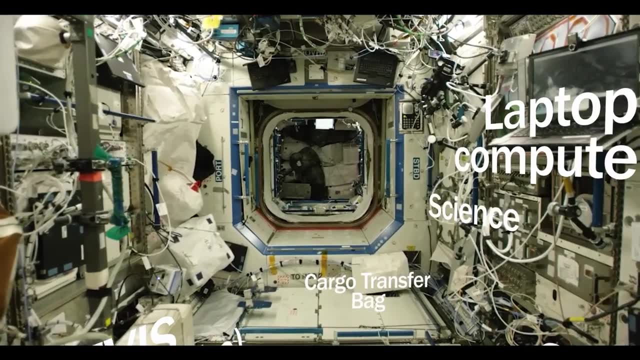 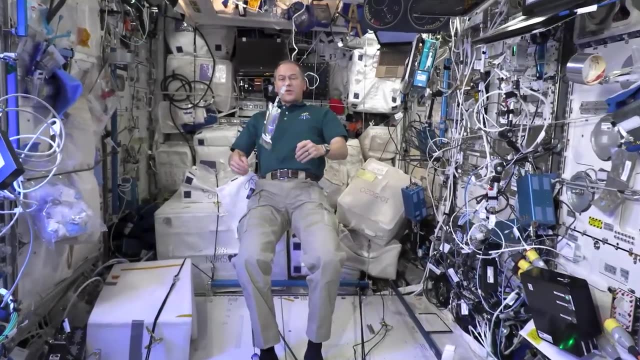 Some of these items are low-tech, like packaging, storage compartments and fasteners. And some of these items are high-tech, like computers, cameras and science experiments. A great example of an engineering solution to something you might be surprised as a problem in microgravity. 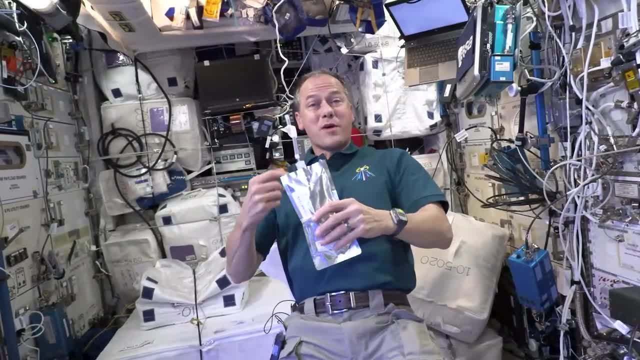 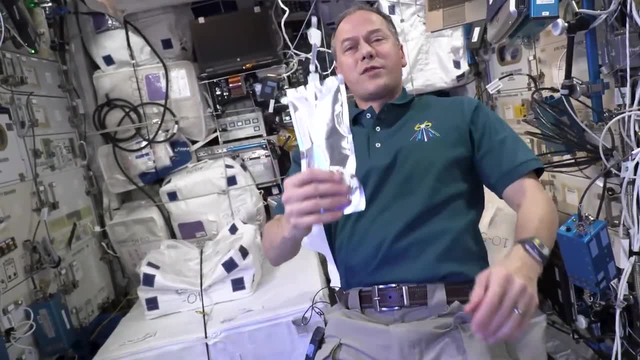 How do we drink fluids, How do we keep them contained And how do we get them in our mouth without making a mess everywhere? Here's our standard drinking pouch. I've got some grape drink in here And a very nicely designed straw. 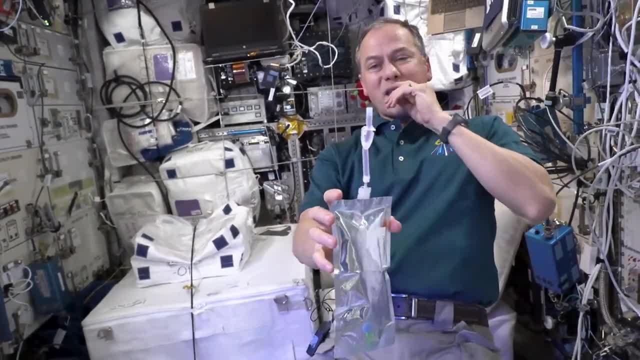 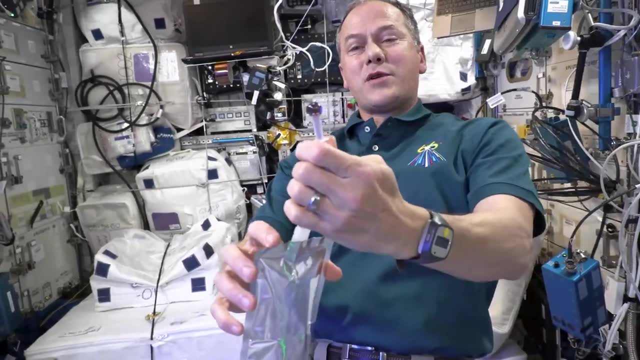 It's just perfect for living in space. If we didn't have this straw, Start to see some fluid coming out there. I don't want to make too big of a mess, so I'm only going to demonstrate what would happen for a second if we didn't have our straw here. 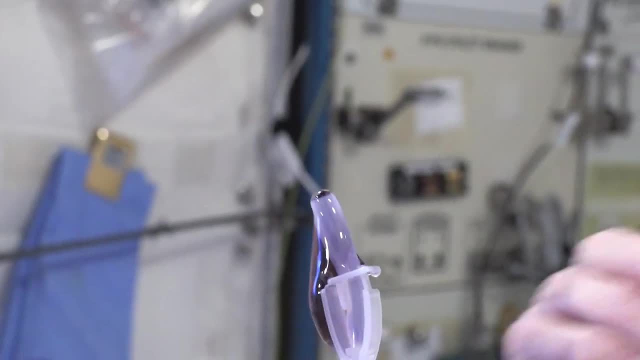 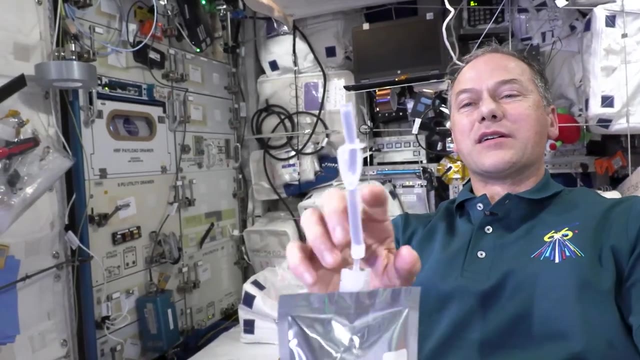 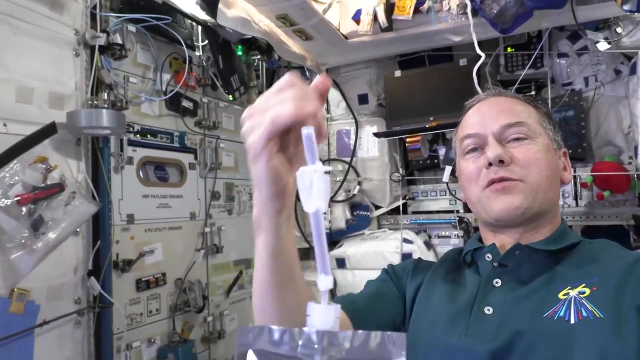 And this would come right off. It's getting on me right now, So let me drink this up. But, as you can see, we have a clasp here, Very nicely designed. It pinches the straw at this point here And that keeps more fluid from coming up the straw. 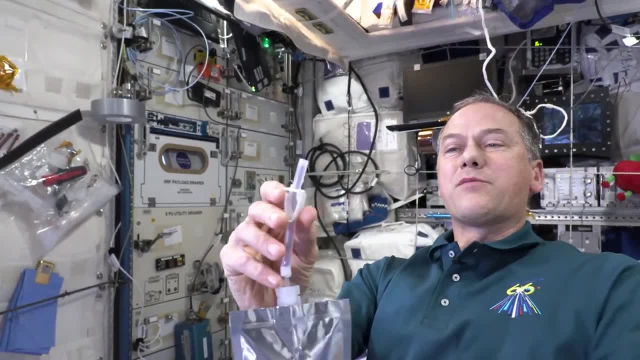 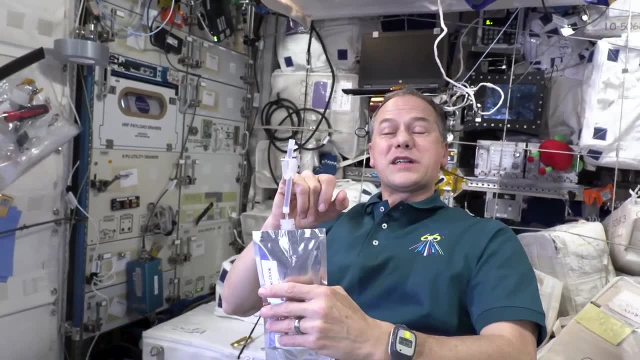 And that way, if you want to drink something, you just open it up. when you need to drink, You have to remember to close it again before you pull it out of your mouth, Otherwise you're going to get more fluid coming out.